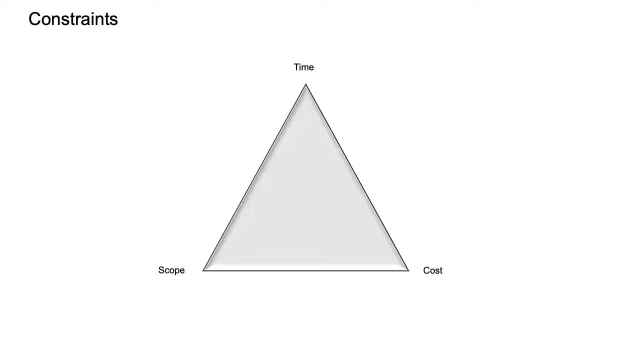 Here comes the most important question: How are you dealing with changes? Do you evaluate constraints and potential impact of these changes? Let's see what contains this process to better understand how it should be treated. But first of all, let's start with constraints Here. think about the kinds of constraints you have in your projects, Or what kind of potential constraints could be in every project. The main constraints which always take place in the project are time, cost, scope. 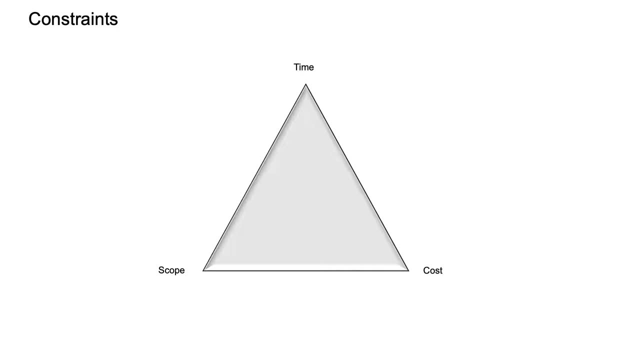 It's called iron triangle or triple constraint. It means that these constraints will always be in your projects. Some of the additional constraints that could appear in the project are quality, risk, procurement, resources, communication. These all are constraints in every project. And now think about some questions. You have planned the duration of the project to be 12 months. 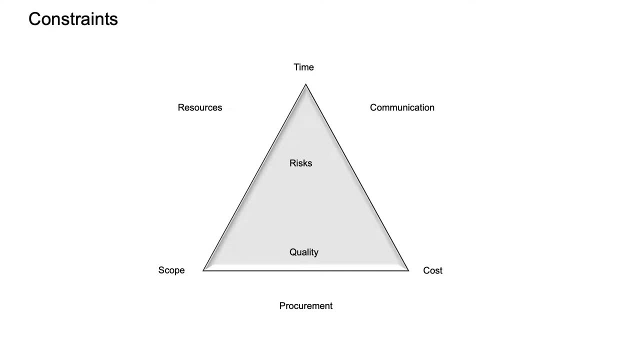 After two months, top management says: Dear team, this project is a strategic one, Therefore it should be finalized in eight months. What will you do next? What is your action plan to finalize this project in eight months? We will have to think how we can compress our schedule to deliver this project in eight months. right, We can use fast tracking or crashing, But let's see the whole flow. 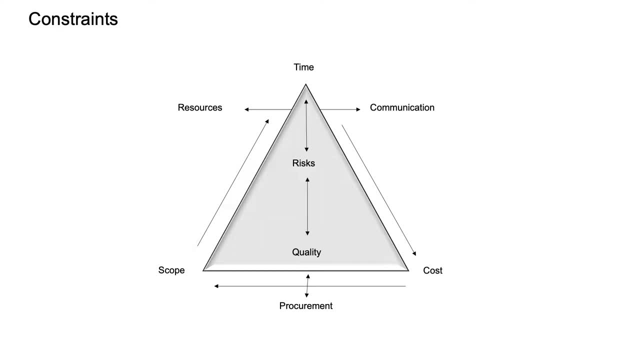 Theoretically speaking, we can crash our schedule. We have to find more money to use for more resources, right Meaning now that we already have two types of constraints: Time, because we need to compress our schedule, And cost, because we have to find more funds for additional resources. For example, we don't have a reserve to hire four more people, but could hire only two additional employees. We will have required quality of this project. 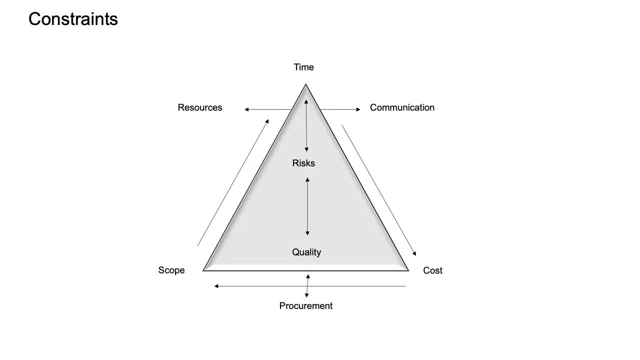 Now we have another constraint: Quality. If we have to compress our schedule, what kind of additional risk will appear? It's a next constraint that will appear: Additional risks: Do we actually have enough people to execute all the required work in time? It's a resource constraint. Probably we could cut something out from this call. This is yet another constraint that has appeared.